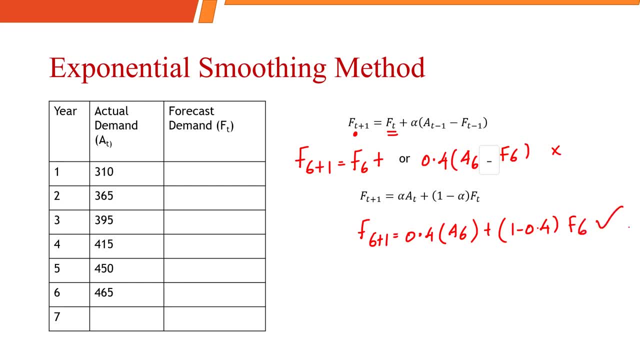 the sixth period. this is more convenient, so i use this particular method. now let's start the calculation. as i have told you, i will be using the second formula for the calculation. alpha can always take a value between 0 to 1.. for the first year, you are given with the demand, but there 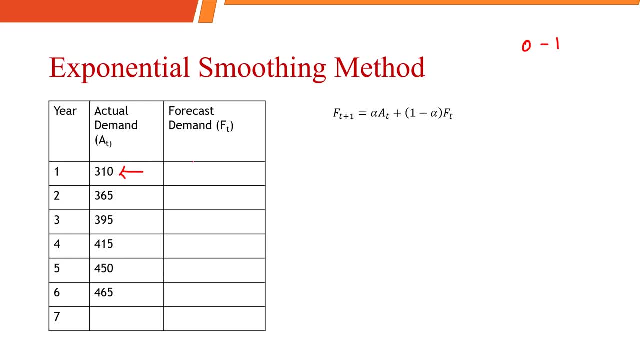 is no change in the demand of the second period as alpha increases from 0 to 1. it is just the same. no forecaster demand without having the previous year demand. it will not be possible in this case. what you can do, whatever is your actual demand straight away, you can post that as a forecaster. 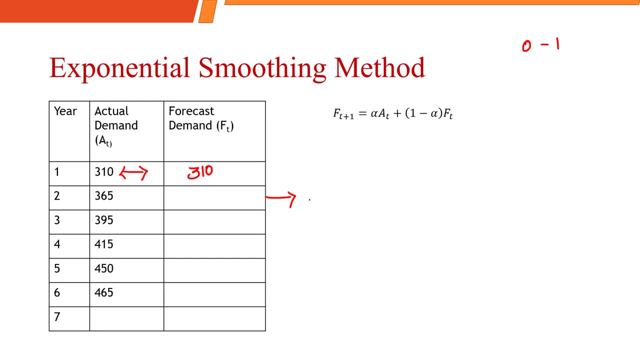 demand starting from period 2 onwards. you can take this for, in this particular given sum we are given with alpha 0.4 and 1 minus alpha is 1 minus 0.4 will give us 0.6. so alpha 0.4, 1 minus. 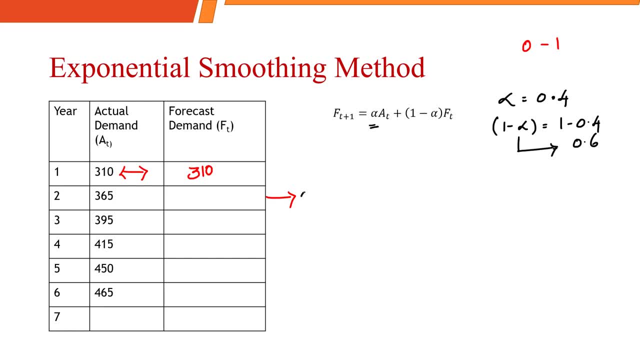 alpha is 0.6. check into it in the formula. we have got an alpha 0.4- actual demand of the previous year: 310 plus 1, minus alpha 0.6 into the forecaster demand of the previous year, 310 0.4 into 310 plus. 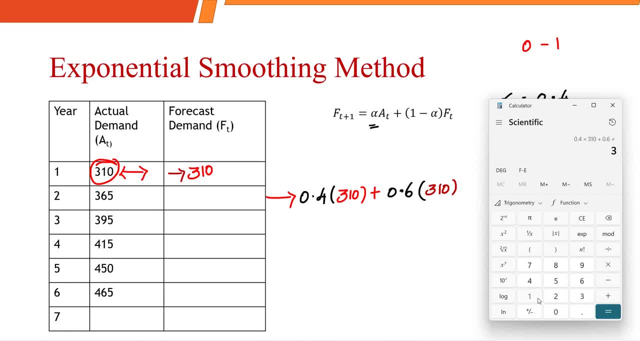 0.6 into 310, you will have a answer of 310. you will have a answer of 310. let's move on to the next calculation. the next calculation is 0.4. what is the demand of the previous year? we are calculating it for. 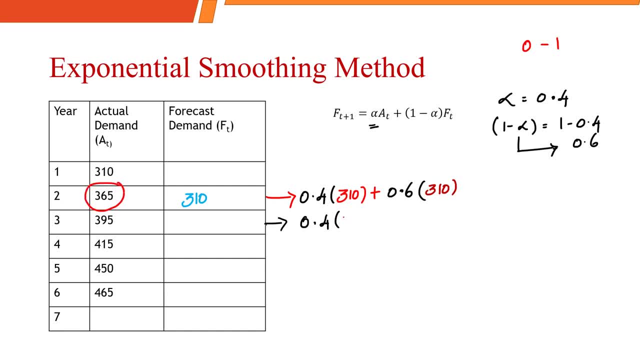 the third year. so the previous demand is 365 plus 1 minus alpha. 0.6 into 310 is the previous forecaster data. 0.4 into 365, 0.6 into 310 gives us a value of 332 to calculate the demand for the next. 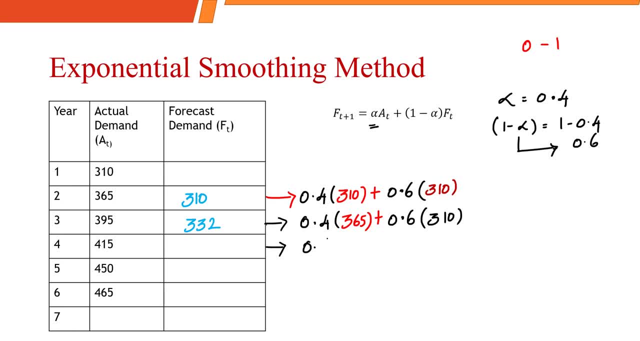 period we are going to take in 0.4 into the actual demand is 395 and the forecasted demand is 332, so we would take 395. the actual demand plus 1, minus alpha, which is whole 0.6, 0.6 into 365, 0.6 into 310, gives us a value of 332 to calculate the demand. 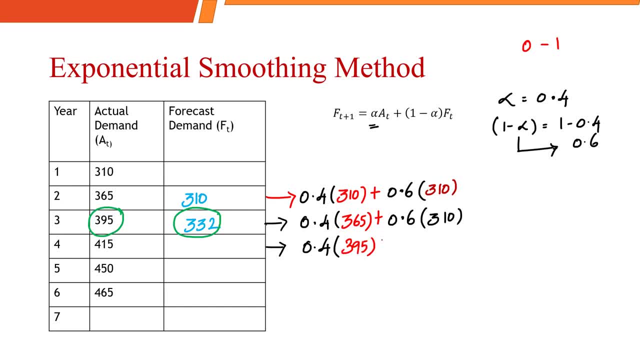 for the next period, we are going to take in 0.4 into the actual demand is 395 and the actual demand is 332, so we would take 395, the actual demand plus 1 minus alpha, which is 0.6, into 310 and the forecasted demand is 0.6, would take 395. 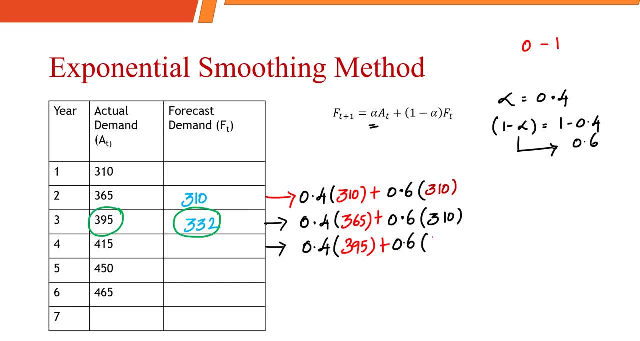 und 53, elevated by rational nodecoding, exerciseangel or bid як way too, have meaning to make this process really easy: 0.6 and the actual demand is 332.. So, which is 0.4 into 395 plus 0.6 into 332. This will give us: 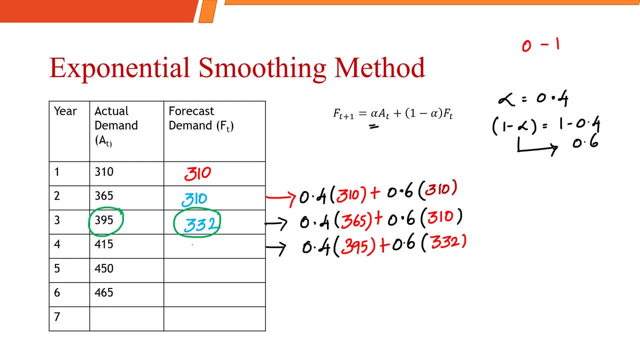 357.2.. So we can round it off 357.. Let's calculate the forecasted demand for the fifth year, which is 0.4 into. the actual demand is 415 and the forecasted demand is 357.. 415: 1 minus alpha. 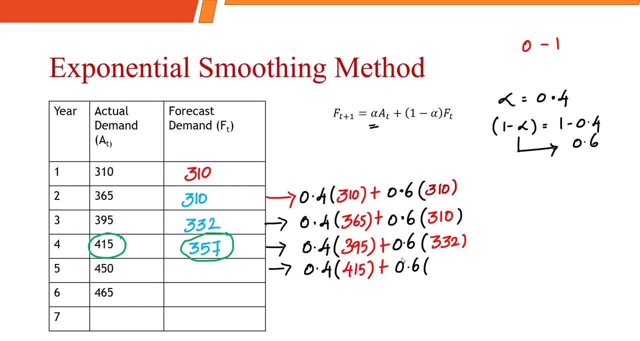 0.6 into the forecasted demand: 357.. 0.4 into 415 plus 0.6 into 357.. This will give us a value of 357.2.. So we can round it off 357.2.. So we can round it off 357.2.. So we can round it off. 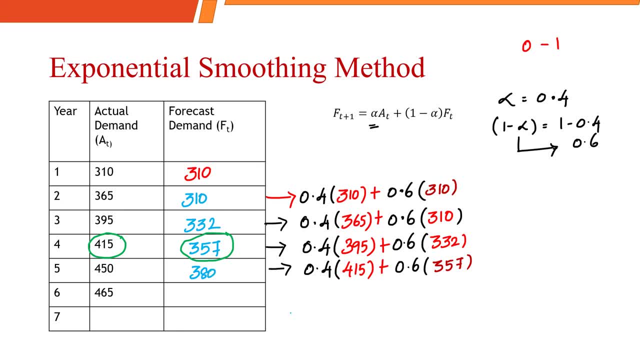 380.2.. 380.. Let's move on to the calculation for the sixth year: forecasted demand: 0.4 into the previous year. actual data is 450 and the forecasted is 380.. So now this becomes 450 plus 1, minus alpha 0.6 into the previous year. forecasted demand: 380. 0.4. 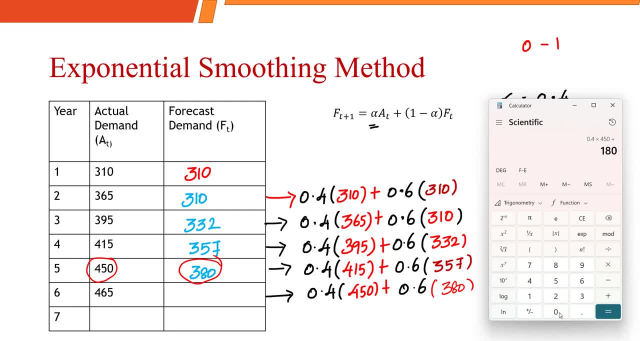 into 415, plus 0.6 into 380.. This would give us 408.. Let's calculate the demand for the last year: 0.4 is the alpha constant. into the previous year demand is 465 plus 1 minus alpha, which is 0.6. 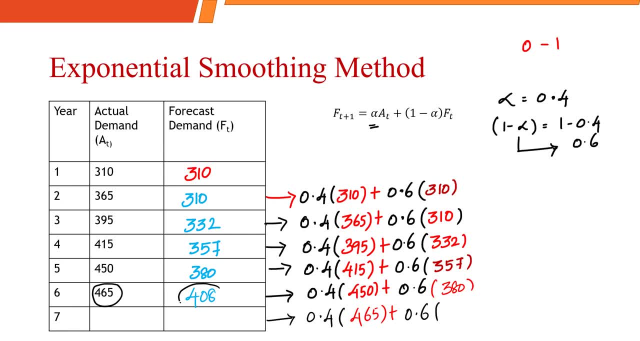 into the previous year forecasted demand, which is 408, which is 480.. So we can round it off 357.2.. So we can round it off 357.2 into 415 plus 1, minus alpha 0.6 into 380.. So we can round it off.